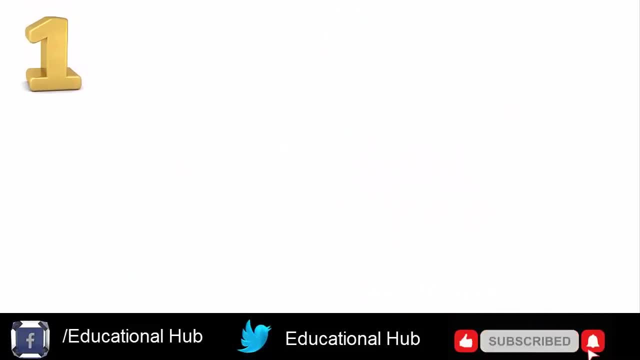 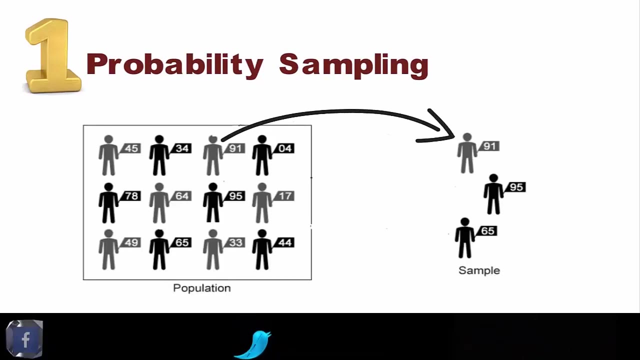 Before choosing specific type of sampling technique, it is needed to decide broad sampling technique. I will shows the various types of sampling techniques. 1. Probability sampling. Probability or random sampling has the greatest freedom from bias but may represent the most costly sample in terms of time and energy for a given level of sampling. 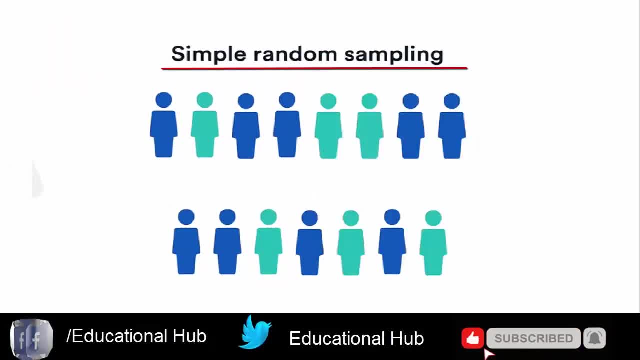 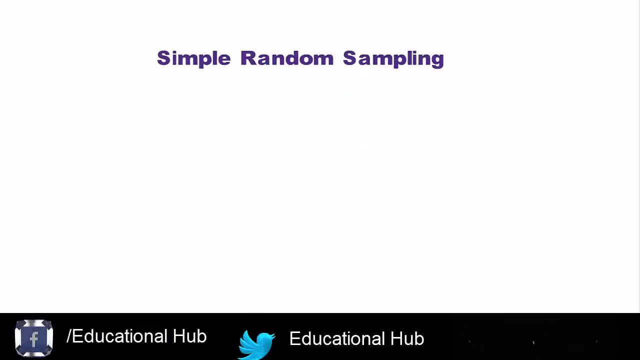 error. 2. Simple random sampling. The simple random sample means that every case of the population has an equal probability of inclusion in sample. Disadvantages associated with simple random sampling include: 1. A complete frame. A list of all units in the whole population is needed. 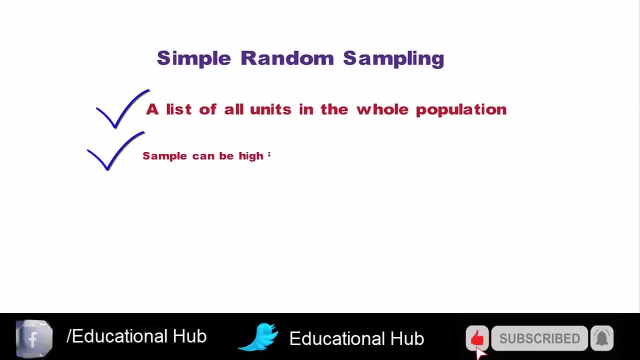 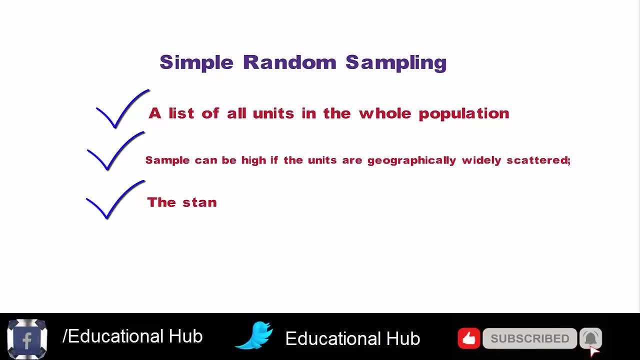 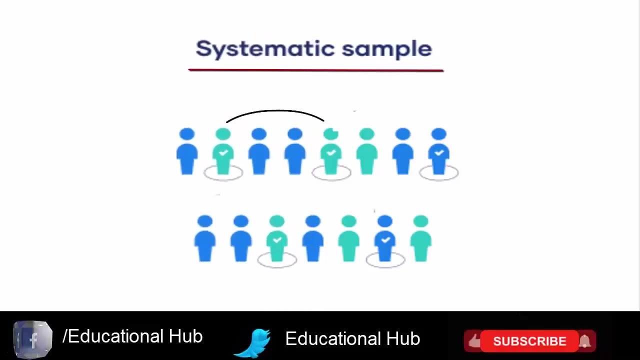 2. In some studies, such as surveys by personal interviews, the costs of obtaining the sample can be high if the units are geographically widely scattered. 3. The standard errors of estimators can be high. 2. Systematic sampling. Systematic sampling is where every nth case after a random start. 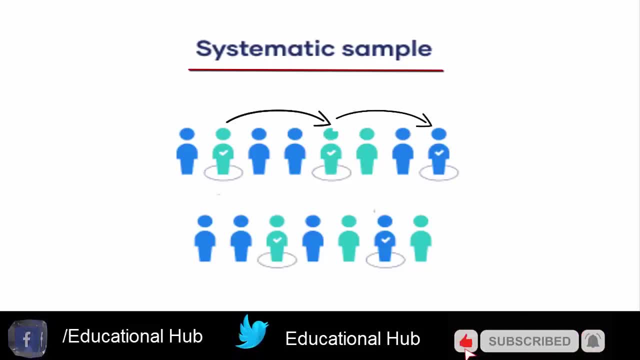 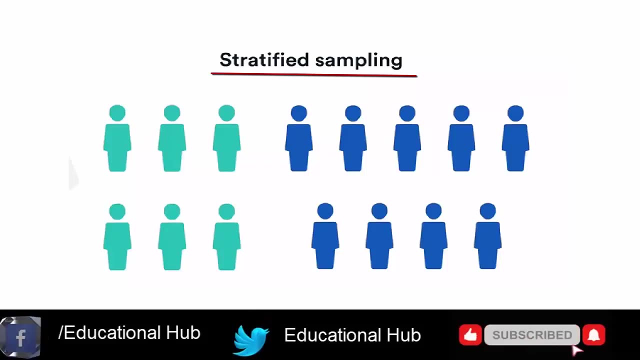 is selected. For example, if surveying a sample of consumers, every fifth consumer may be selected from your sample. The advantage of this sampling technique is its simplicity. 3. Stratified random sampling. Stratified sampling is where the population is divided. 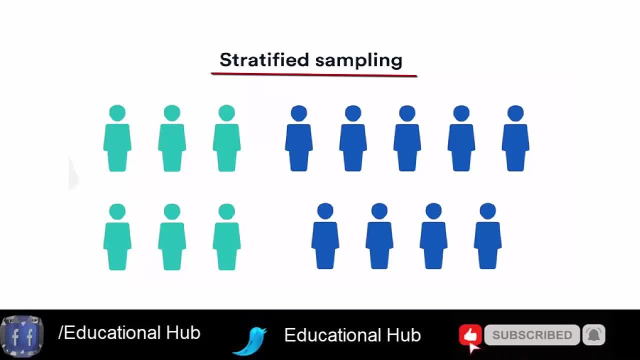 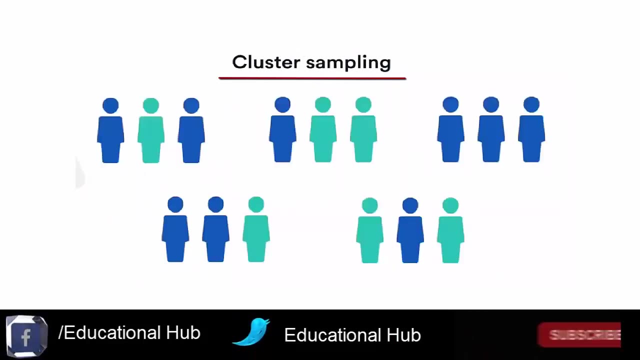 into strata or subgroups, and a random sample is taken from each subgroup. A subgroup is a natural set of items. Subgroups might be based on company size, gender or occupation. 4. Cluster sampling. Cluster sampling is where the whole population is divided into clusters or 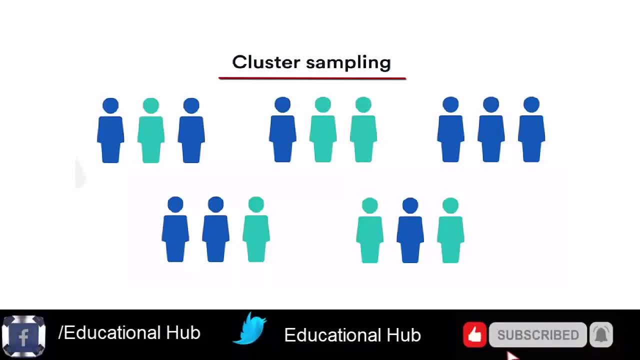 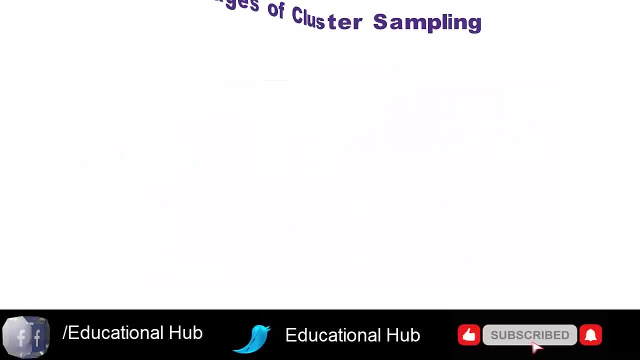 groups. Subsequently, cluster sampling is advantageous for those researchers who are not related to the group. For example, cluster sampling is where you divide between different groups and the groups are grouped in three groups. You can do cluster sampling for study or forzier or forger or forger, and you can do some other types of numbers. 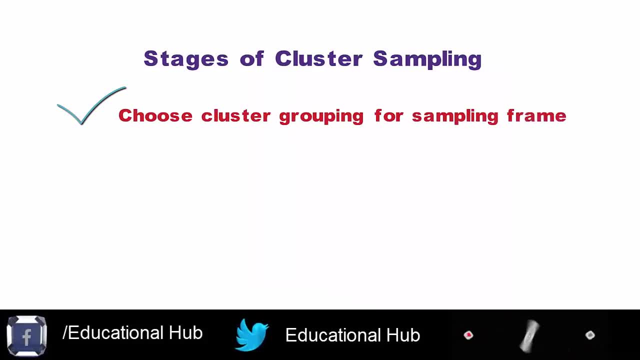 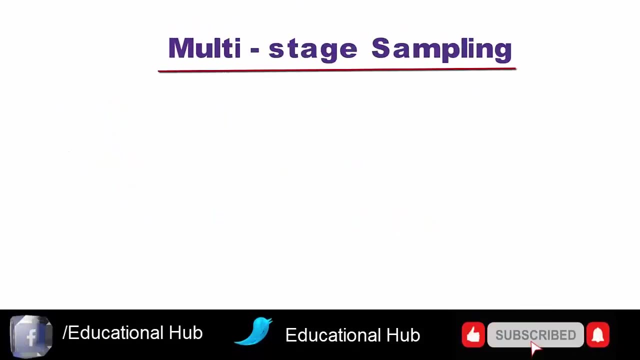 1. Choose cluster grouping for sampling frame, Such as type of company or geographical region. 2. Number each of the clusters. 3. Select sample using random sampling. 5. Multi-stage sampling. Multi-stage sampling is a process of moving from abroad to a narrow 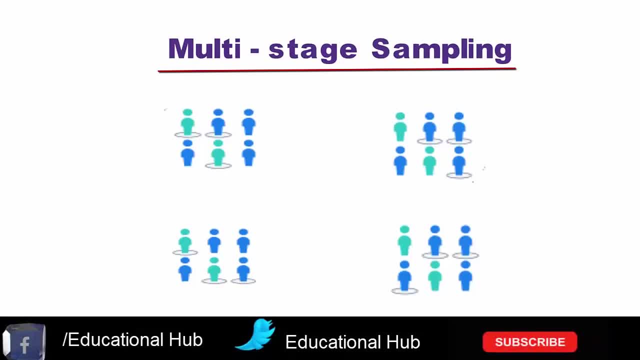 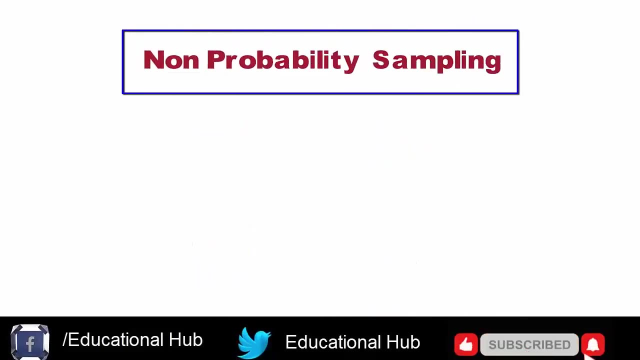 sample using a step-by-step process. if, for example, a american publisher of an automobile magazine were to conduct a survey, it could simply take a random sample of automobile owners within the entire american population. two: non-probability sampling. non-probability sampling is often associated with case study research, design and qualitative research. with regards to the latter, 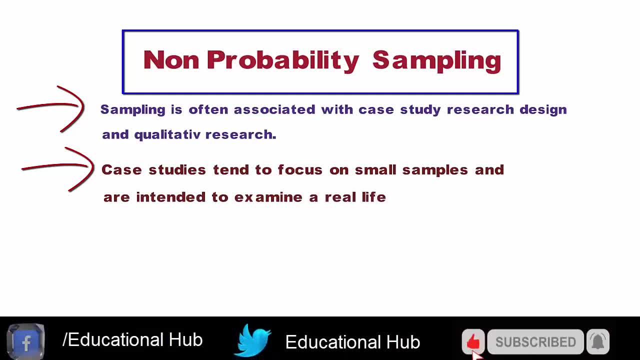 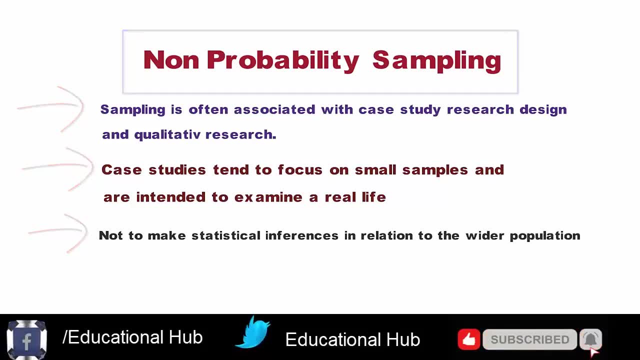 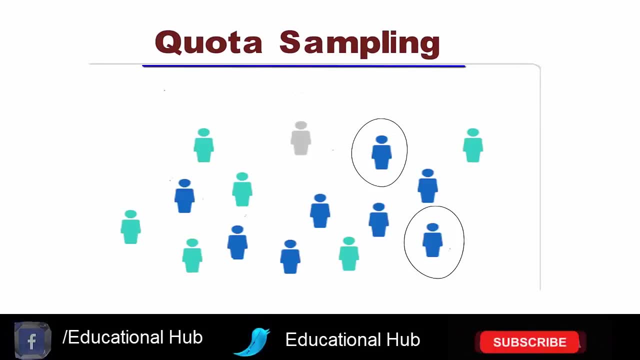 case studies tend to focus on small samples and are intended to examine a real-life phenomenon, not to make statistical inferences in relation to the wider population. one quota sampling. quota sampling is a non-random sampling technique in which participants are chosen on the basis of predetermined characteristic so that the total 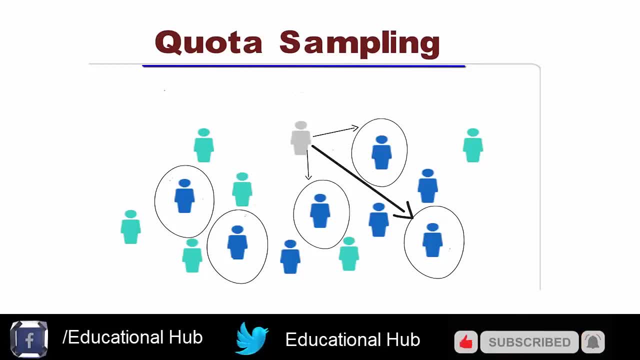 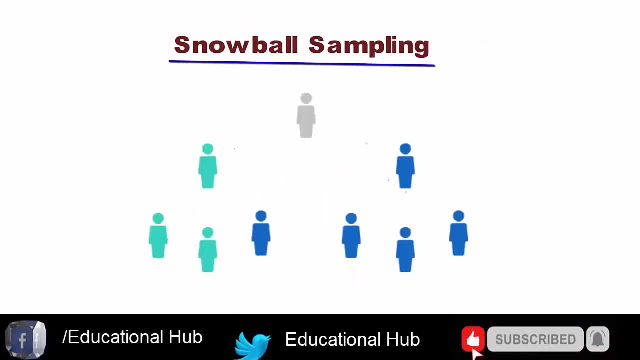 sample will have the same distribution of characteristics as the wider population. two: snowball sampling. snowball sampling is a non-random sampling method that uses a few cases to help encourage other cases to take part in the study, thereby increasing sample size. this approach is most applicable in small populations that are difficult to access due to their closed. 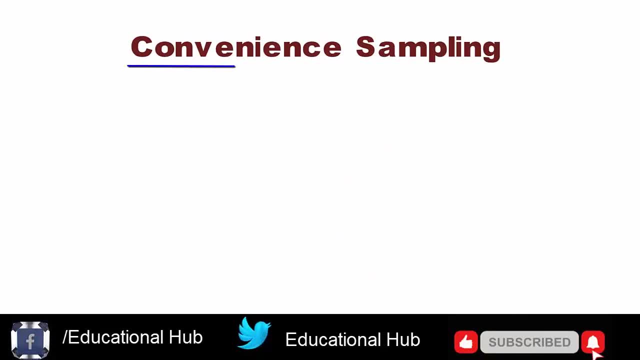 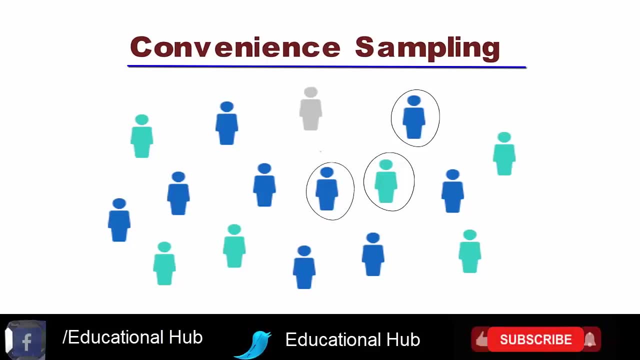 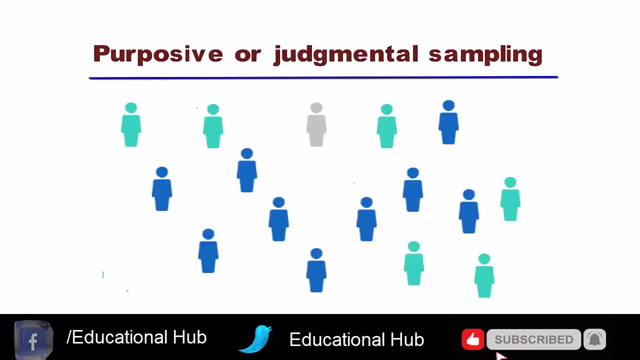 nature. three: convenience sampling. convenience sampling often helps to overcome many of the limitations associated with research. for example, using friends or family as part of sample is easier than targeting unknown individuals. four: purposive or judgmental sampling. purposive or judgmental sampling is a strategy in which 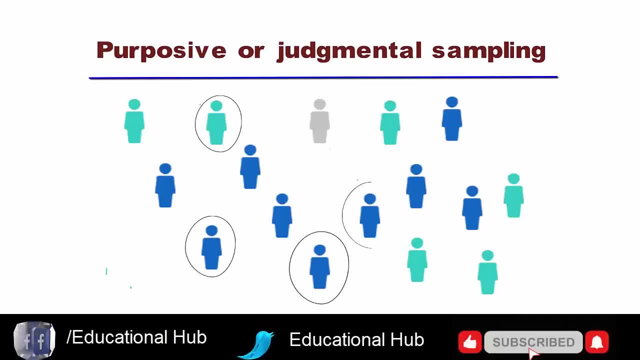 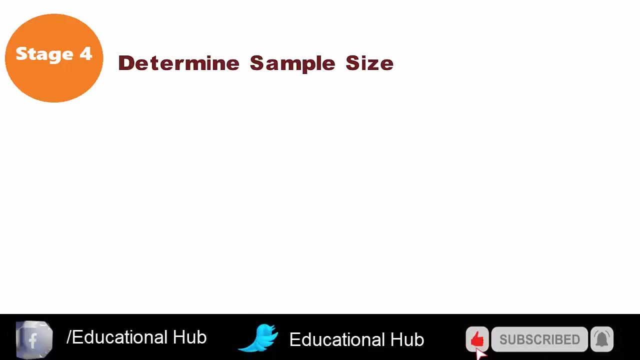 particular settings, persons or events are selected deliberately. it is where the researcher includes cases or participants in the sample because they believe that they warrant inclusion. stage four: determine sample size. in order to generalize from a random sample and avoid sampling errors or biases, a random sample needs to be of adequate size. what is adequate depends 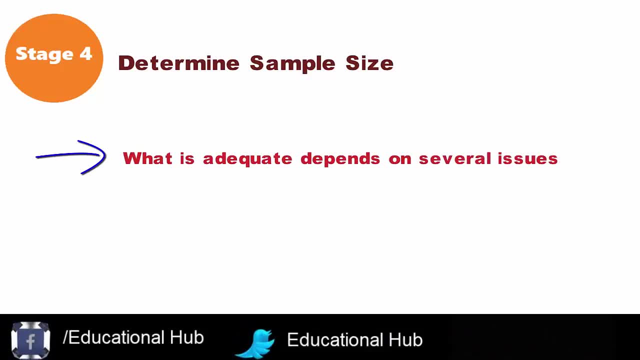 on several issues which often confuse people doing surveys for the first time. this is because what is important here is not the proportion of the research population that gets. there are numerous approaches incorporating a number of different formulas for calculating the sample size, for categories of sample sizes or by the size of the sample size for.